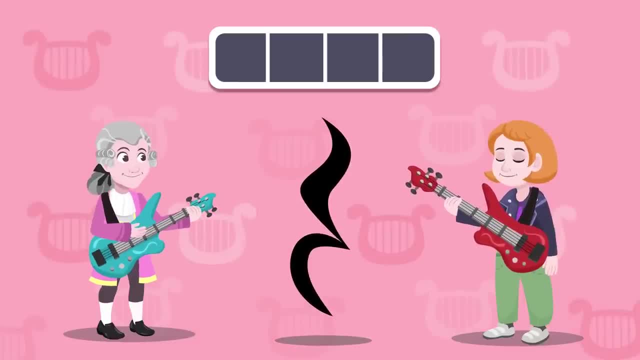 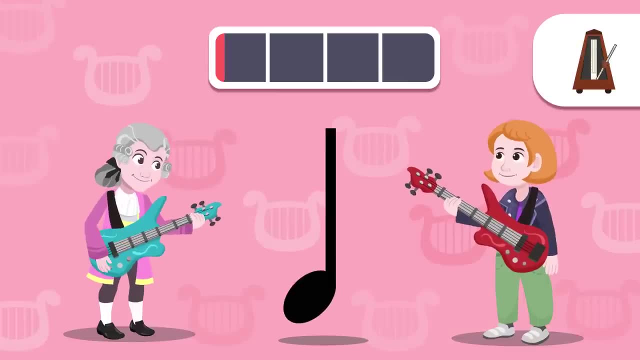 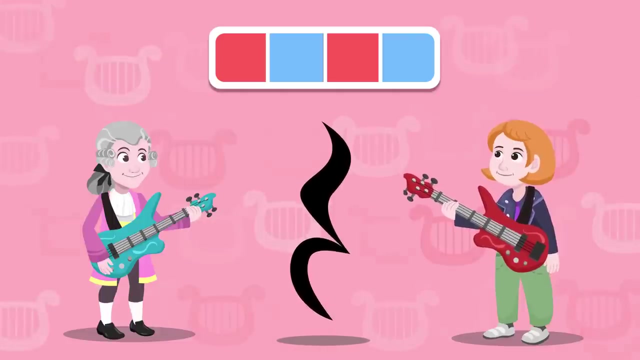 Rest notes are just as important as sound notes and also last a certain amount of time. Should we try it again? Let's go for it. What did you think of the quarter note and its rest note? Now I am going to explain the half note. 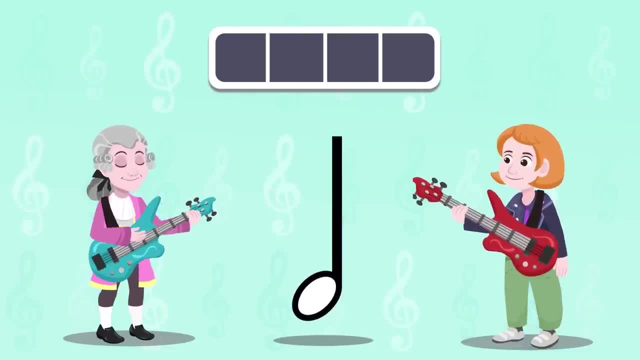 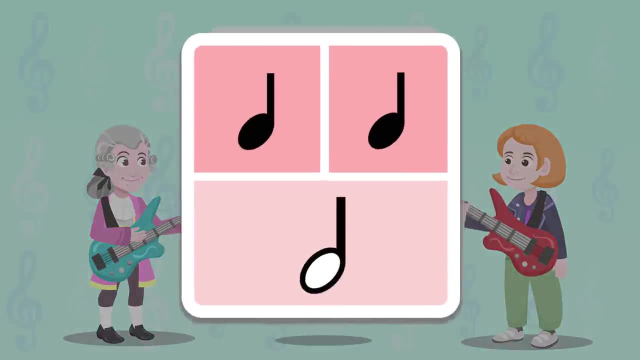 This is the half note. It's the same shape as the quarter note, But if you look closely you will see that the head is not black. How else are they different? Instead of being one beat like the quarter note, it has two beats. 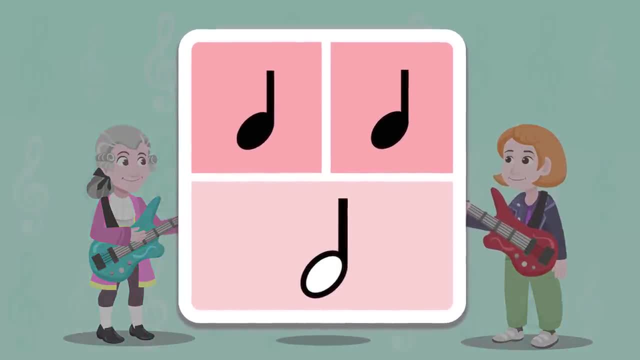 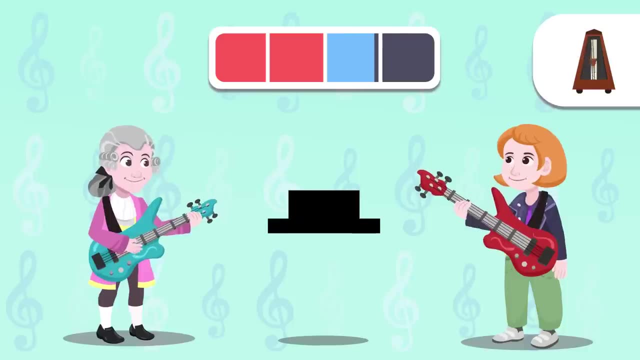 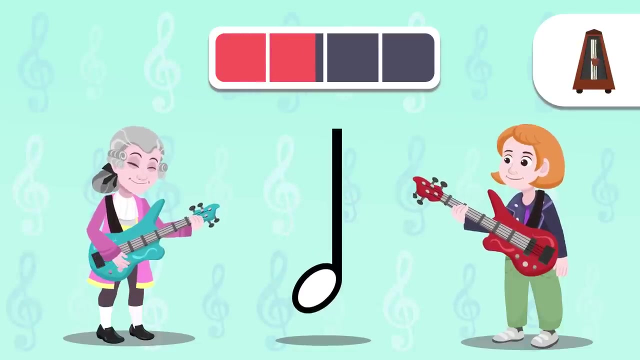 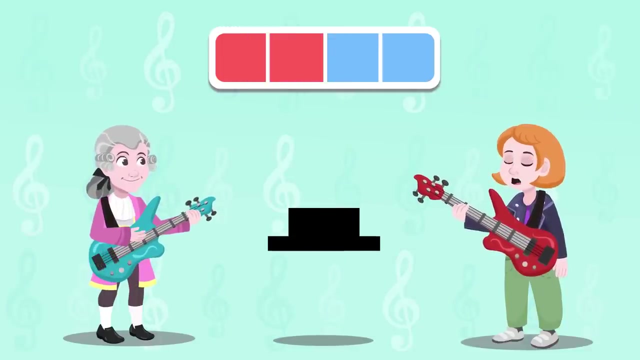 Basically, one half note equals two quarter notes. Let's take a look. So when we see that little hat, when there's complete silence, it's a half note. rest, right, That's right, my friend. This one here is a whole note. 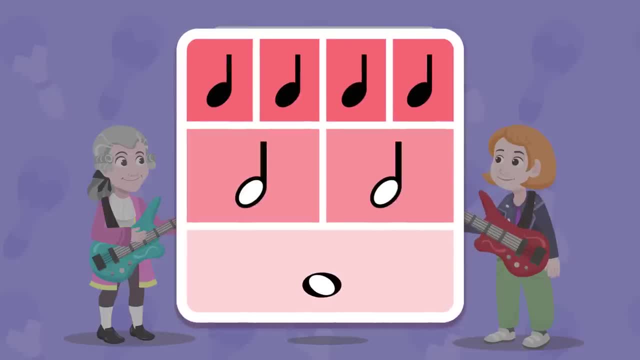 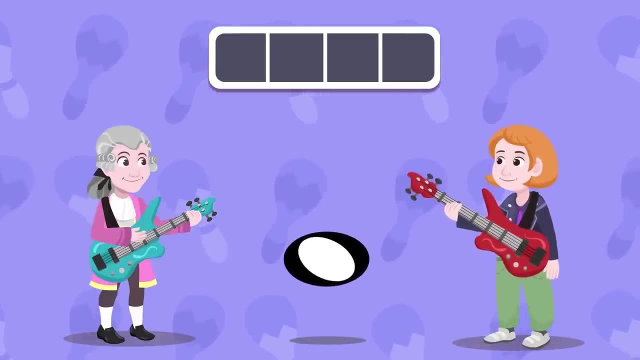 It is equal to four quarter notes and two half notes. Wow, It lasts for a really long time. Yeah, It has four beats. Listen, Get ready, because I am also going to show you the rest. beat, Rest beat, Rest beat. 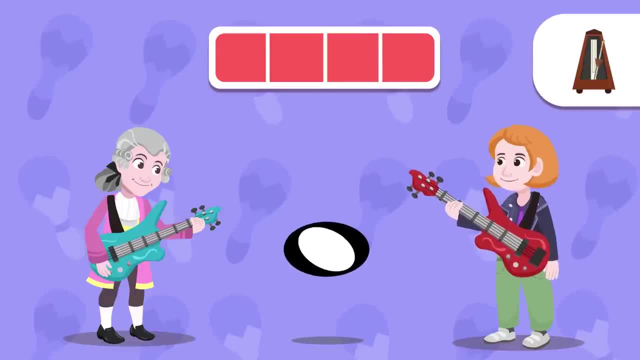 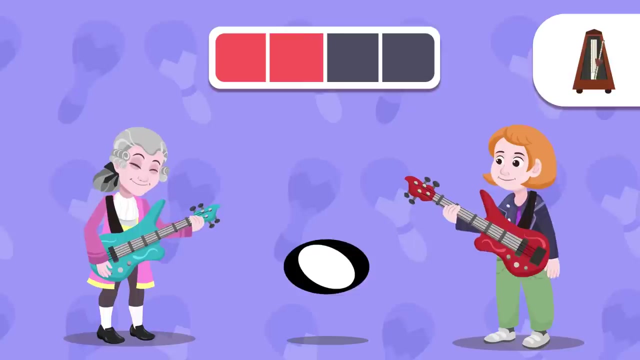 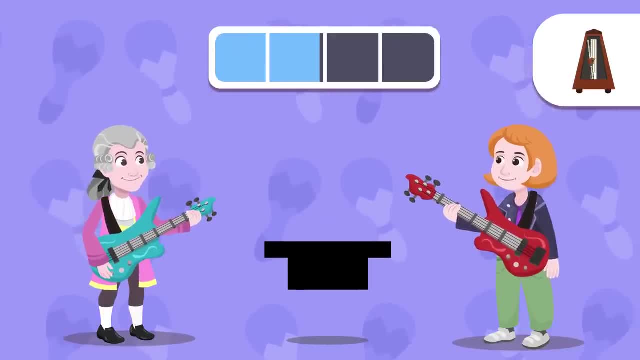 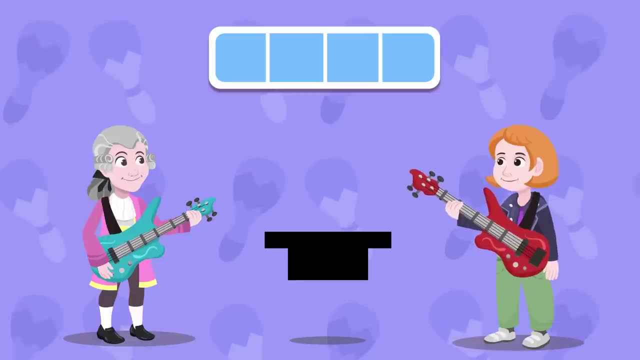 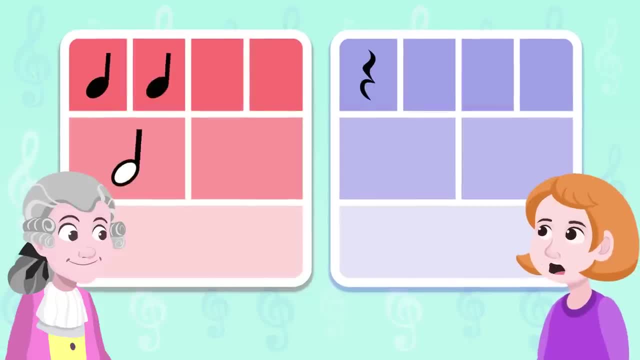 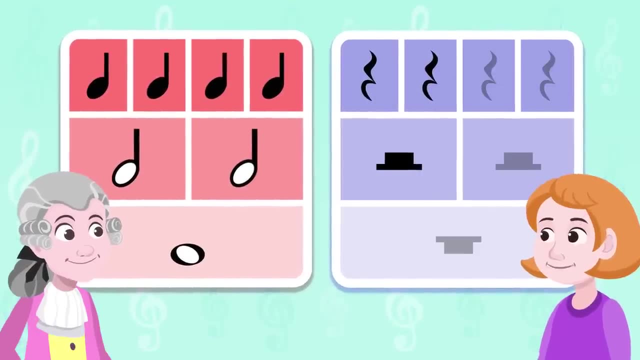